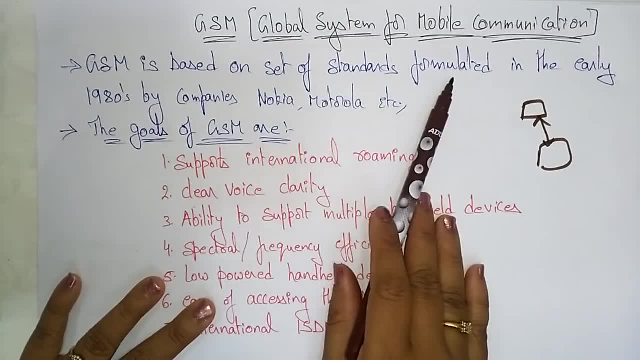 explain the thing. GSM is based on the set of standard formulated in the early 1980s by companies Nokia, Motorola and Ericsson. So many companies are there, So all those companies is formulated in the early 1980s. So all those companies are there. So all those companies are there. So all. 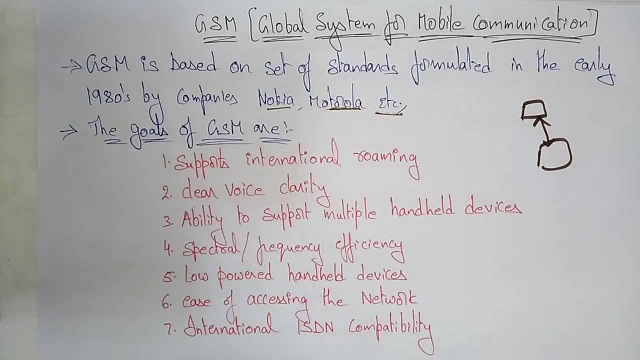 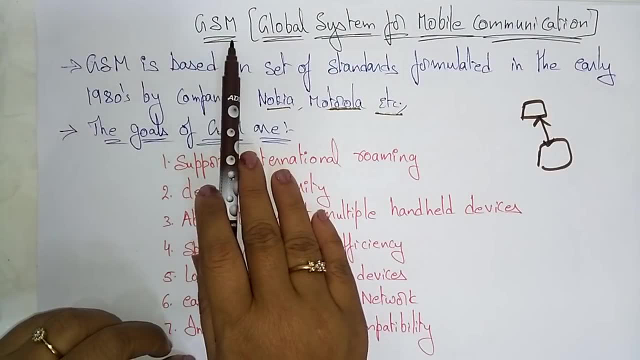 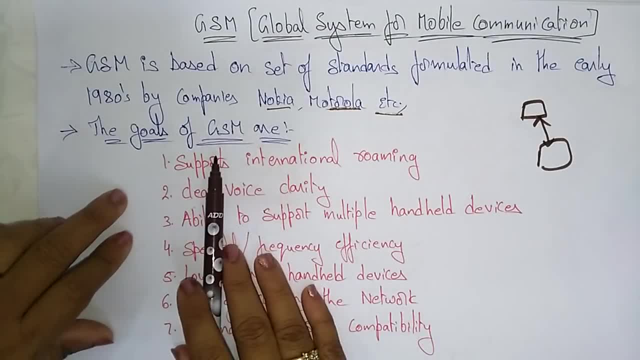 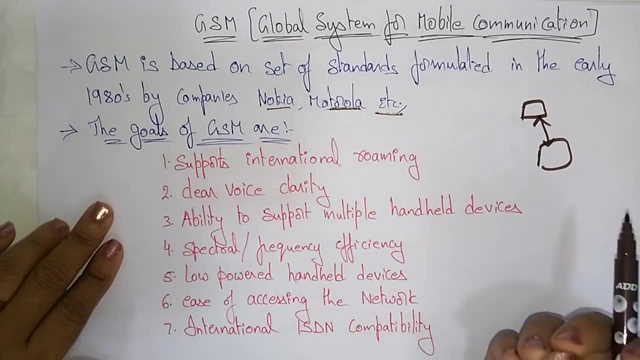 Global system mobile communication. The main goals of GSM are: supposing international roaming, Suppose your mobile is having the GSM facility, GSM ship is available for you. you can use your mobile phone in any mobile device-building environment. Okay, intentionally one mobile phone. another country. also. it supports the international roaming, international roaming facility. the clear voice clarity. with the help of this global system for mobile communication that is a GSM service you are having, the voice of communication will be clear. ability to support multiple handheld devices. spectral or frequency efficiency will be there. low powered handheld devices. ease. 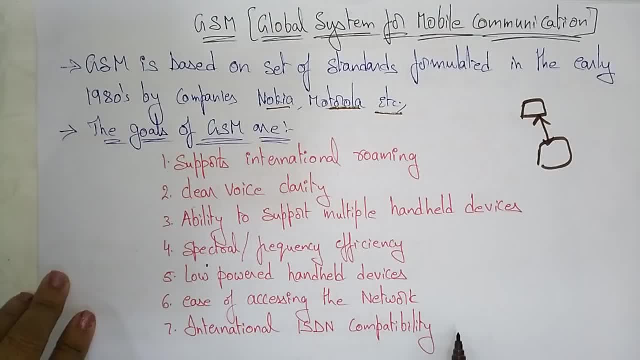 of accessing the network, international ISDN cap compatibility. so these are all the goals of GSM. so by seeing these girls, what goals, what you understand. the main use of this global system for mobile communication is used for the voice clarity and for international roaming and for international ISDN. 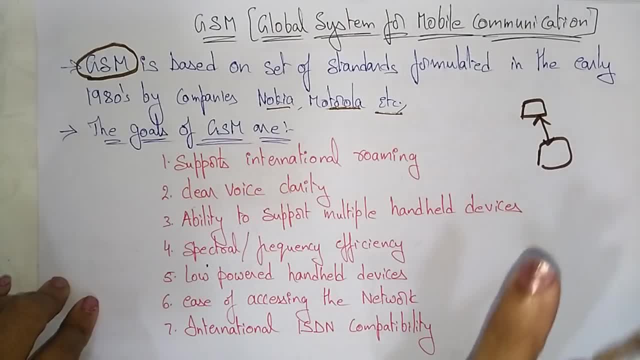 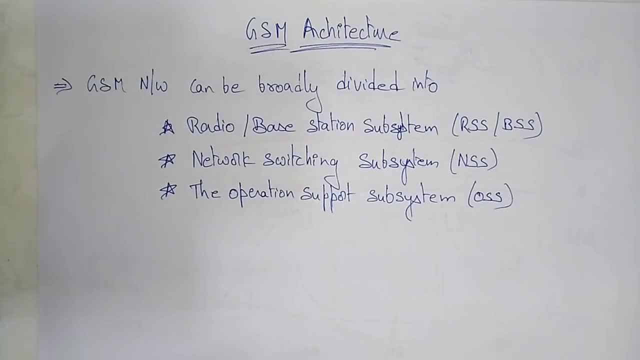 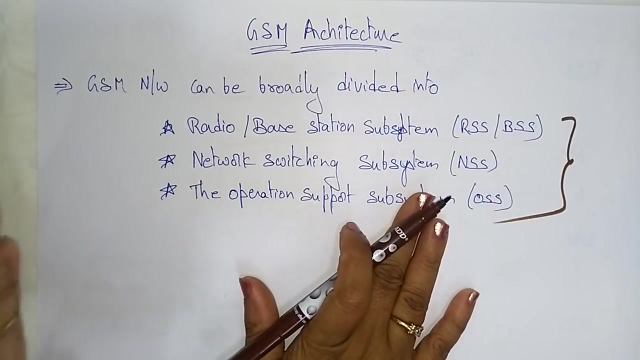 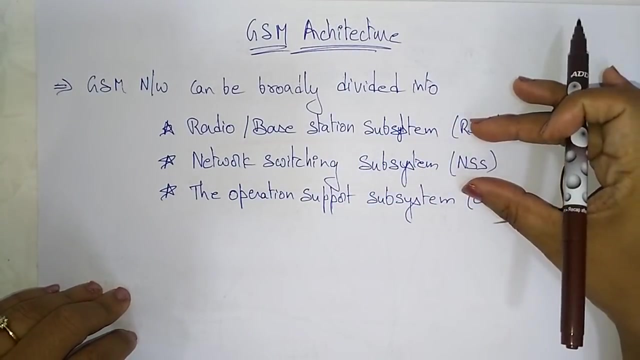 compatibility and ease of accessing networks. we are using the global system for mobile communication. now let's see the architecture. the global system, mobile communication architecture, that is, a network, can be broadly divided into main three. the complete architecture is divided into three subsystems. okay, so complete, this is the GSM. the GSM consisting of these main concepts. one is the radio or base station subsystem are, as as radio subsystem networks, is switching subsystem and operation support subsystem. the complete GSM is divided into radio subsystem, network switching subsystem and operation support subsystem. okay, so radio base station subsystem. so for receiving the signals from the base stations, this RSS will be useful and the network switching. 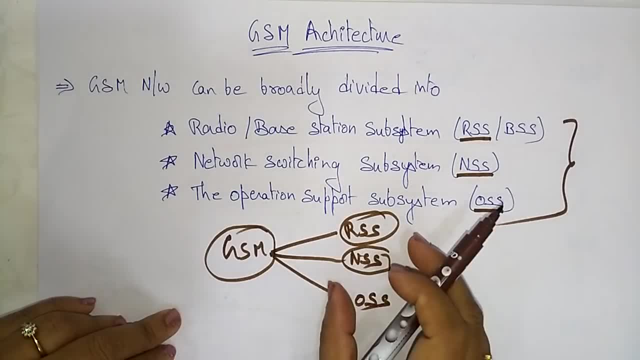 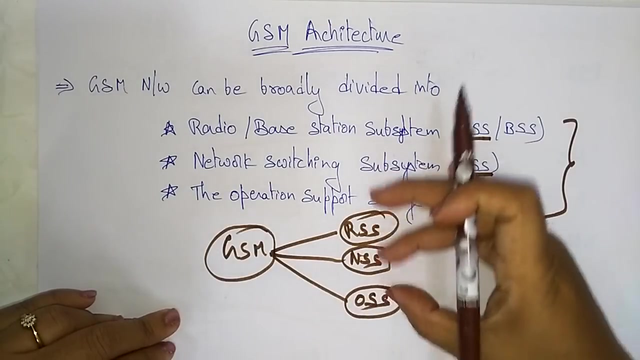 subsystem. if you want to switch the network from one network to another network, the gsm is using the network system switching subsystem and oss is dealing with the operational support of the subsystem. means whatever the mobile device that you are using, that complete operational setup will be handled by the operation support subsystem. so the complete gsm is based on these three. 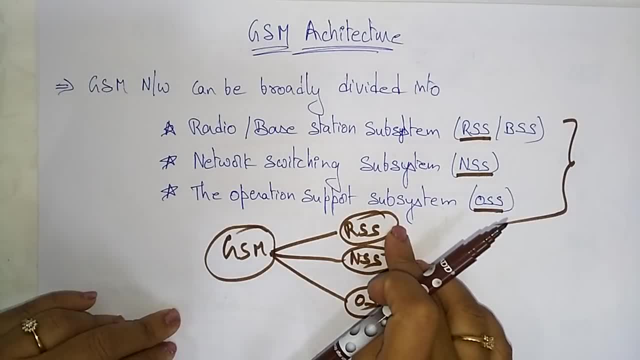 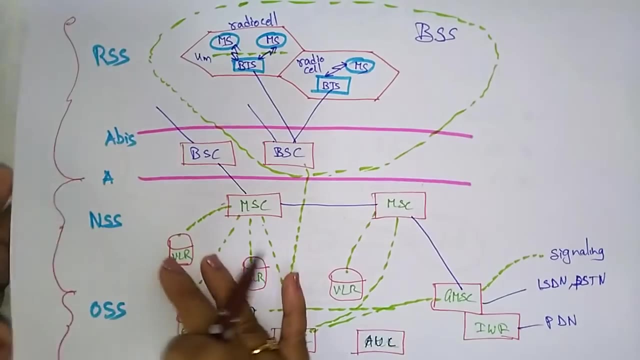 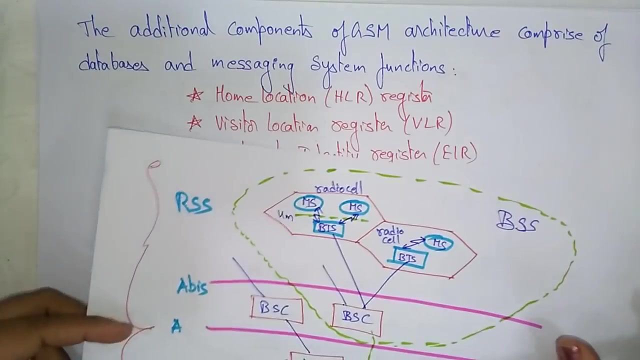 subsystems. so it requires the radio subs, radio station subsystem, network switching subsystem, the operation support subsystem. so just remember these three subsystems. now let's see the architecture. so here this is an architecture general view, architecture view of gsm: here the additional components of gsm architecture comprises of databases and messaging system. 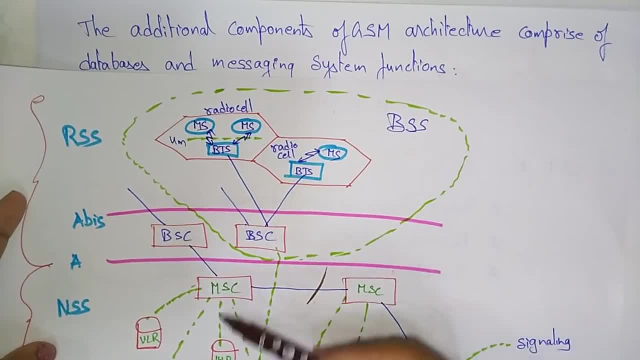 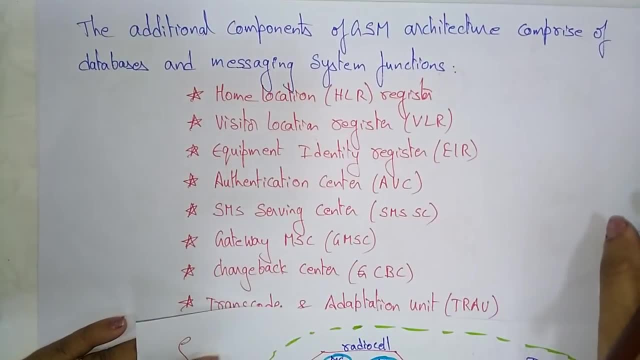 flow and the gsm architecture is a system that is used for the operation of gsm functions. so, whatever the terms that you i used here, the abbreviations, so those i have written here, hlr means home location register. i already explained what hlr will store. hlr is a database. 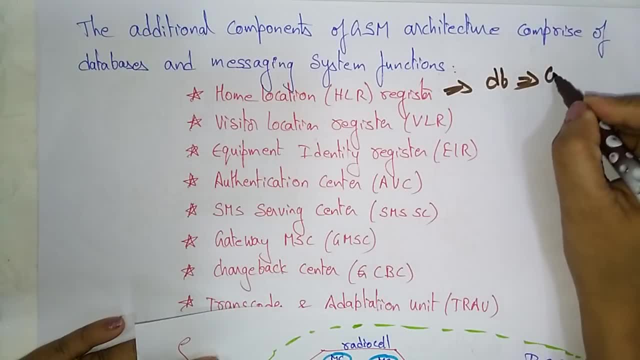 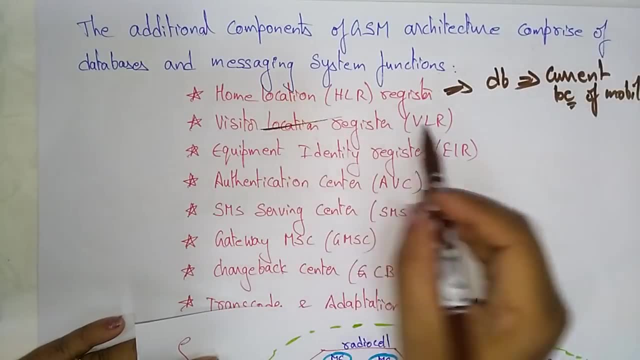 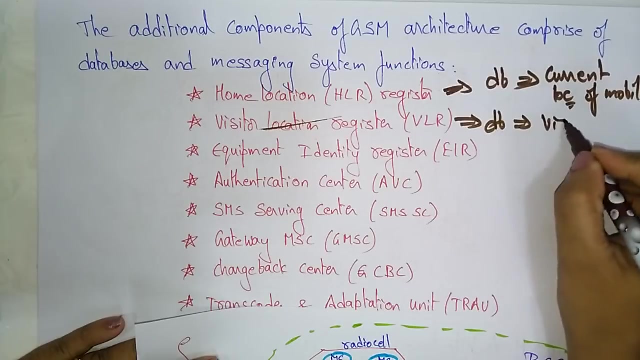 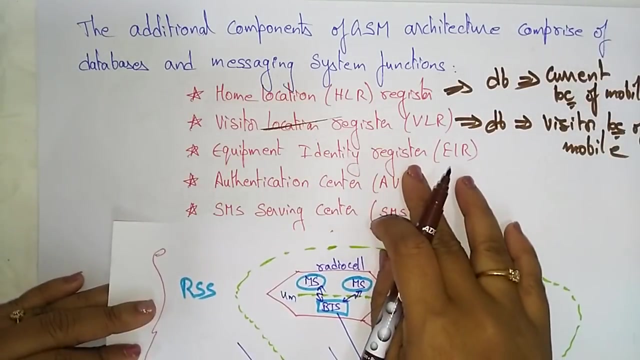 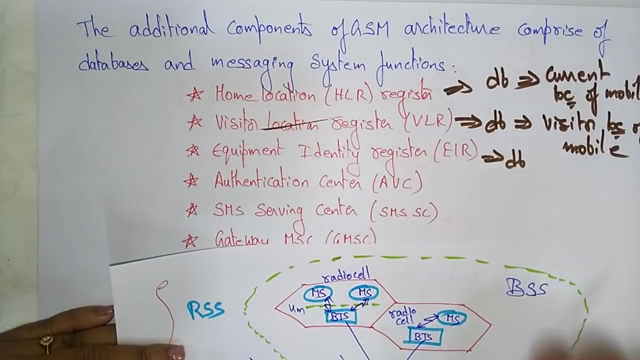 user to store the current location of the mobile, current location of mobile device, whereas visitor vlr. vlr means visitor location register. it is also a database. it stores the visitor location, visitor location of mobile and equipment id register. the equipment id register is also a database. this is used to store the equipment regarding what type of mobile you. 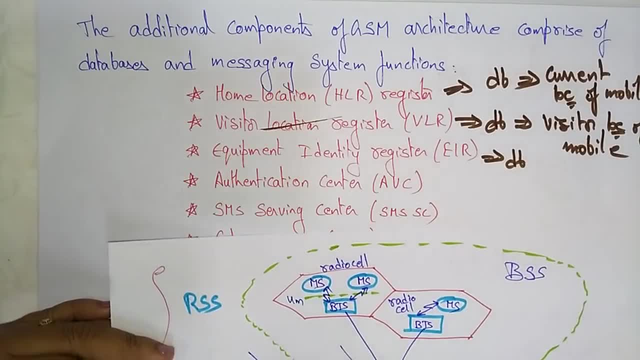 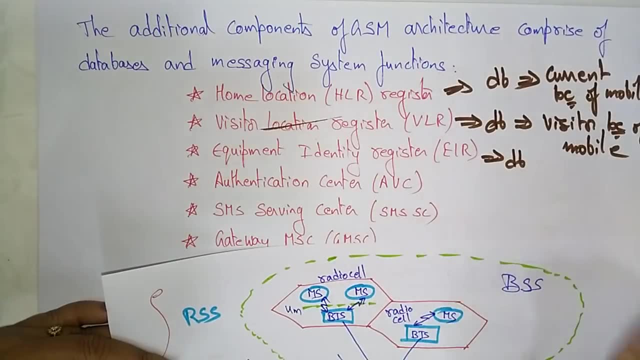 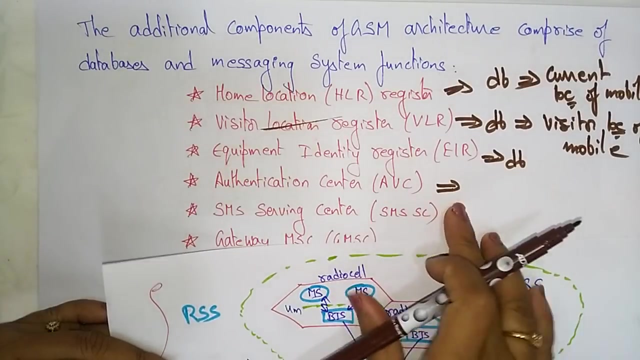 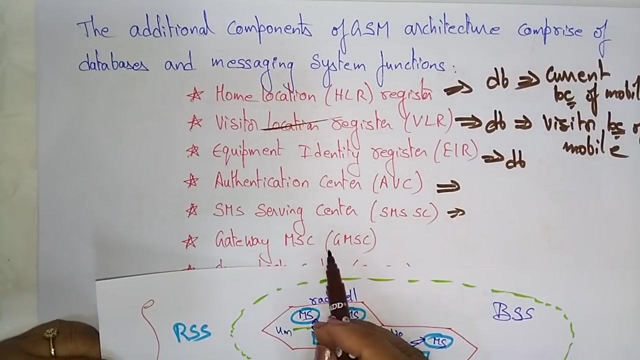 are having and what ip mobile is. having means, suppose, if your mobile is missed or it was theft by someone, by using this equipment identity register you can find out where your mobile was missed. so that is, that is a our Wolfeduckkkhold so soon. 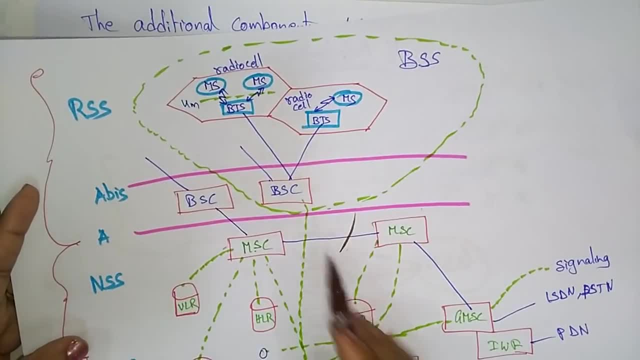 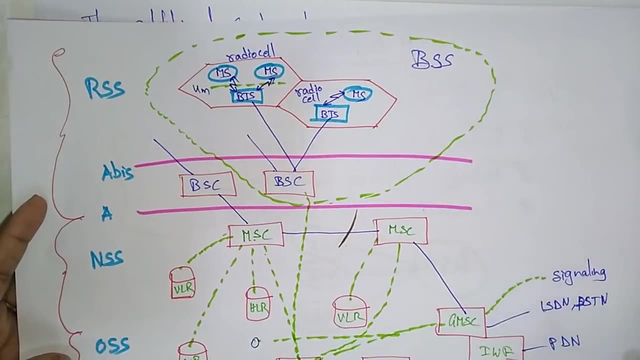 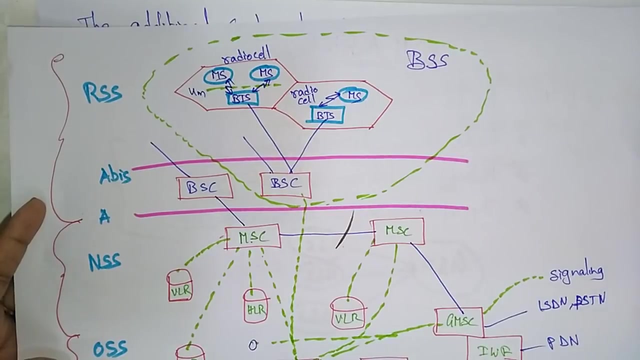 switching center. so i you already know that mobile switching center, so all mobile switching centers will be connected to one gateway will be there in between the mobile switching center and the external uh public switch telephone network there is a gateway connection will be there so that i already explained how the database user, the user device, mobile, will be connected to the. 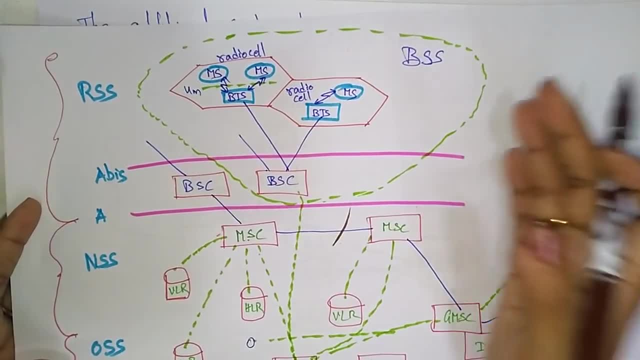 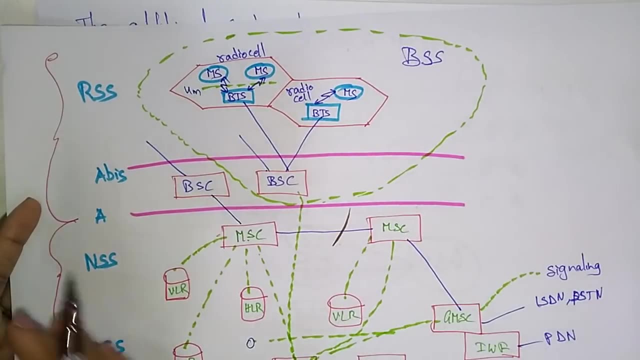 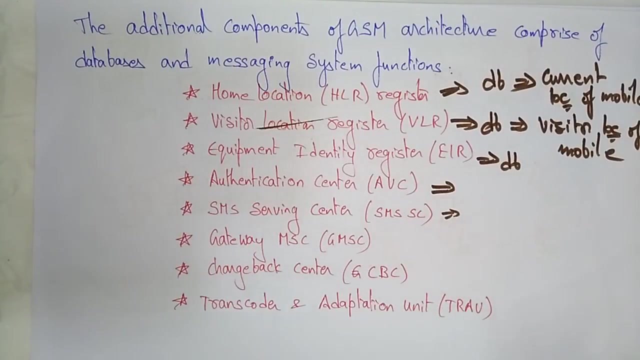 public switch telephone network. with the help of the middleware and with the help of this gateway, you are communicating. with the help of the network, you are communicating the voice or data, whatever it may be okay. and uh, charge back centers, transcoder and adaption unit. now let's see the. 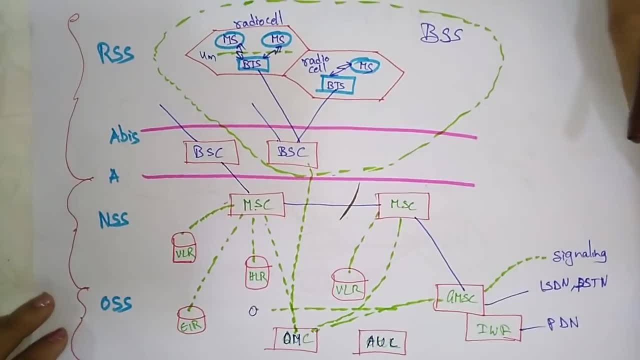 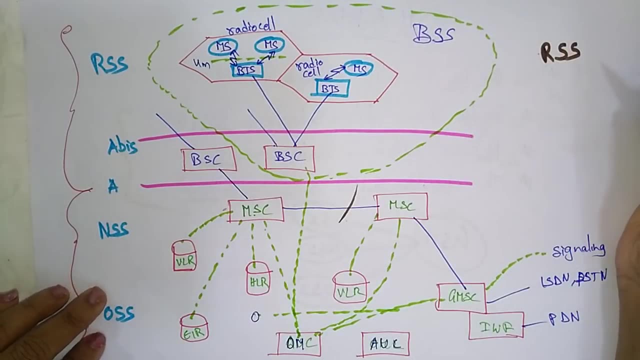 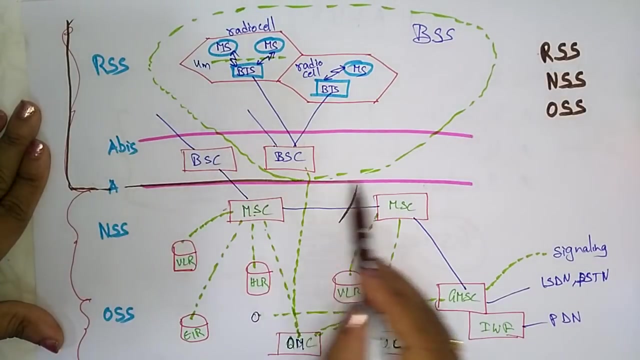 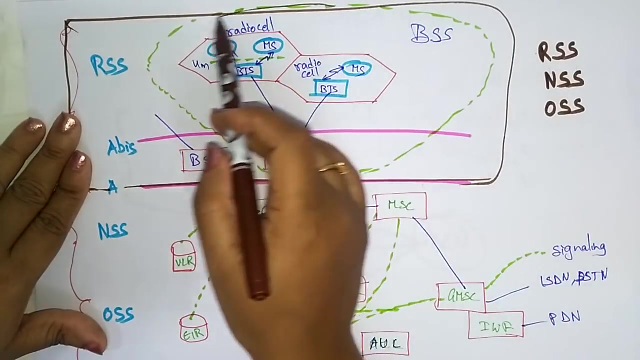 architecture. so what i said? the complete gsm architecture is divided into three subsystems: radio sub system- okay, radio station subsystem, network switching subsystem and operational switching subsystem. so this is a complete structure. so what this radio station subsystem consisting of? so up to here, this is a radio station subsystem. it's, let's take this is a coverage area, so in each, a cell will be there. 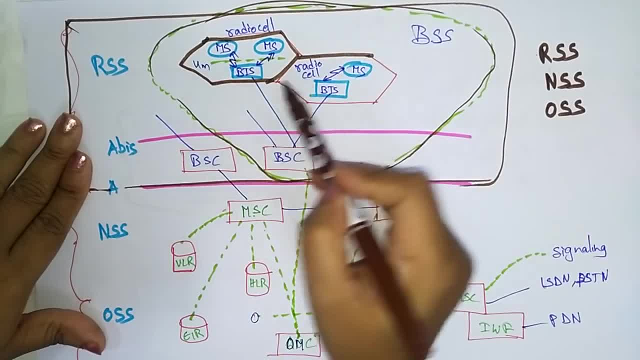 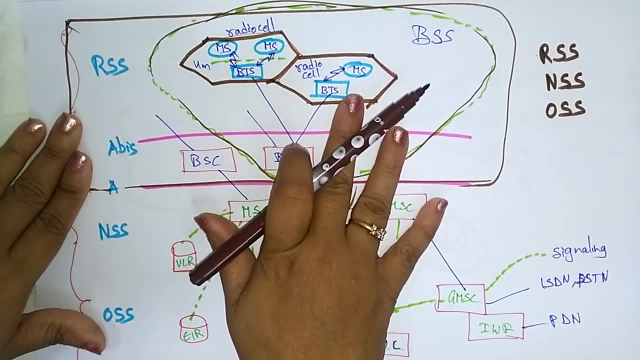 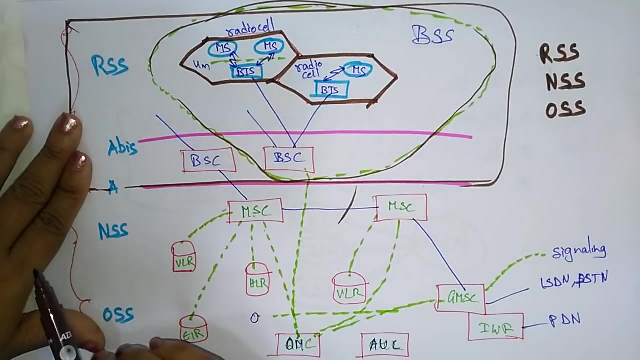 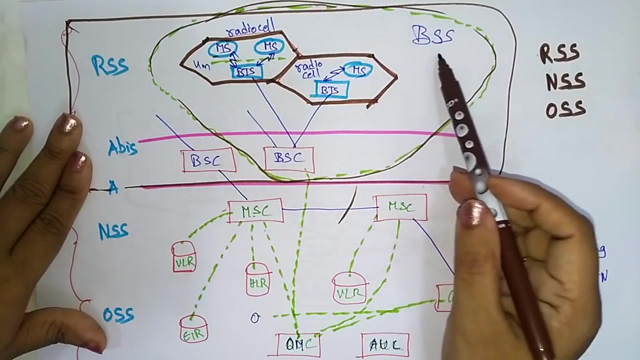 so what i said? the cell consisting of base station, that is, a transmitter which transmits and receives the signal. so there is cells will be there, that is, the radio cells will be there. so each radio cells is having the base stations. okay, the mobile stations will be there, okay, and bss. so what i said? the bss is the uh, base station, base switching. 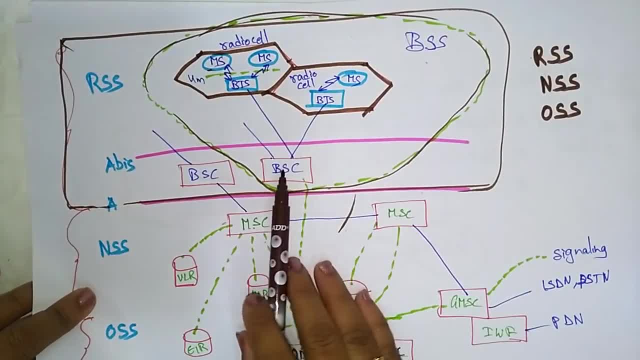 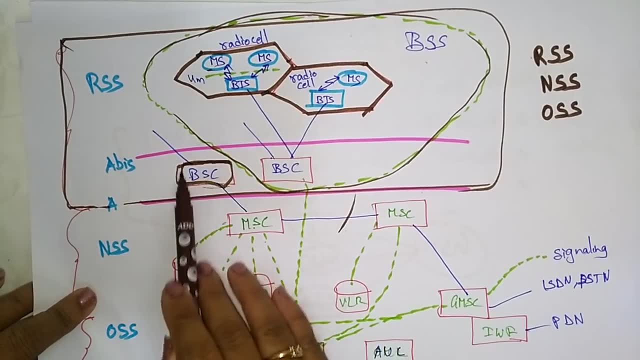 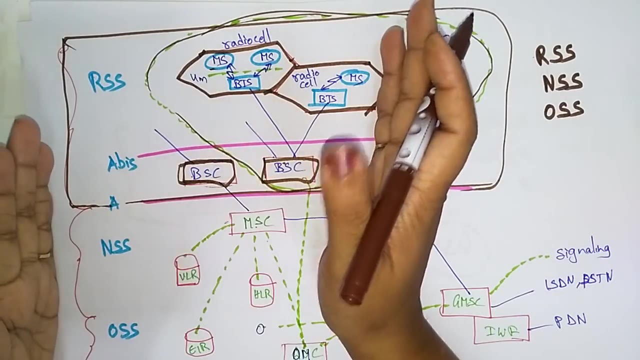 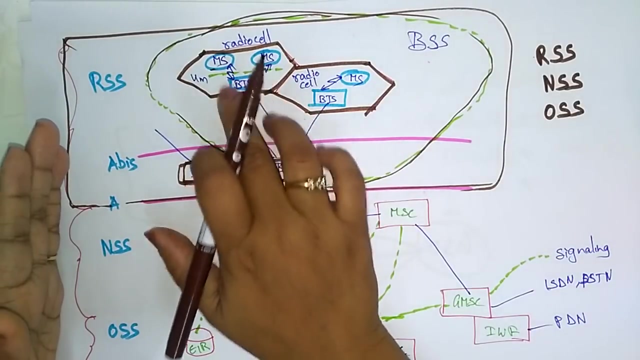 center and base switching circuit controller. you second, base base station controller. this is bsc is a base station controller. so just remember that the radio cells consisting of the different cells, each radio cells is having their own base station. bts means base station, that is, having the base station. 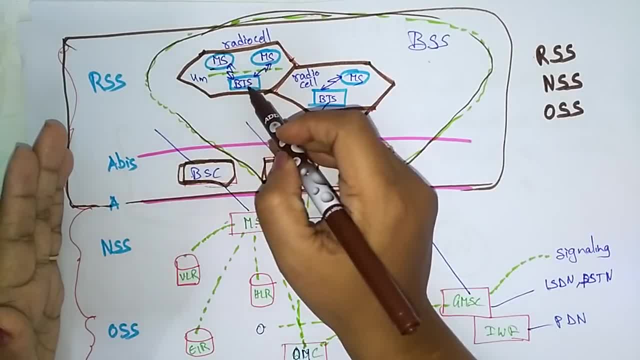 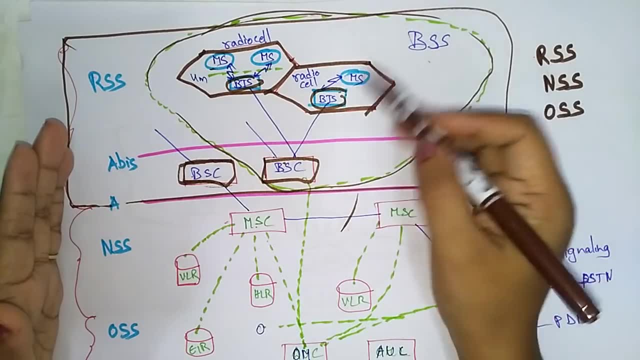 a base station will be connected to the mobile services. so there are e. this base station is connected to two mobile services and this base station is connected to one mobile services. let us take so many mobile services will be connected. each base station is handling one mobile services. 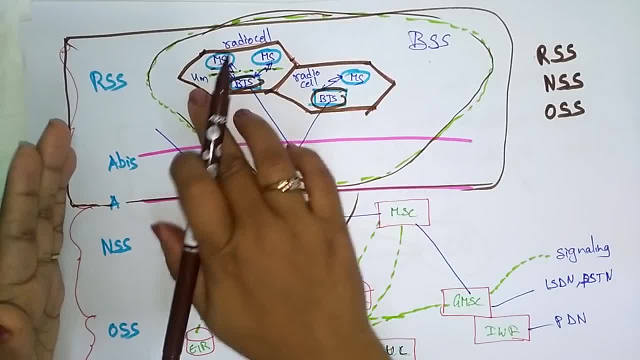 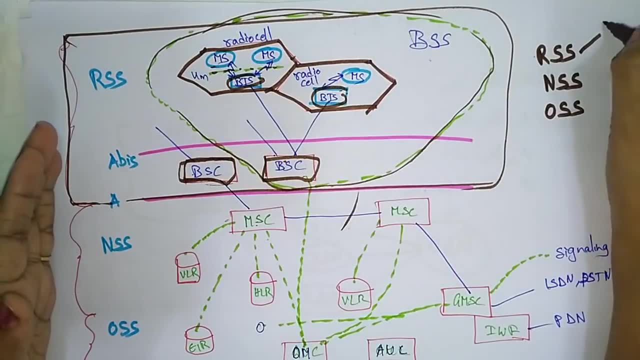 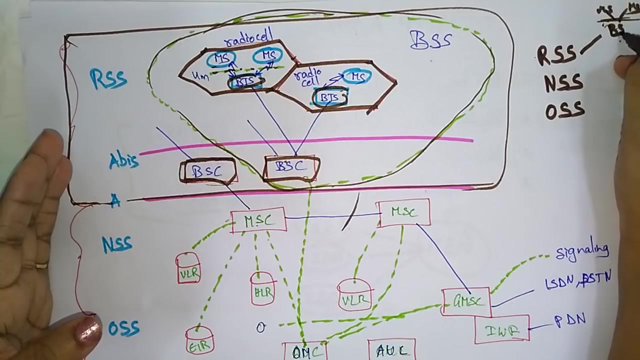 so in between the mobile services and the base station there is an interface will be there. um interface will be there. remember that rss is going to connect it as a base station. each base station connects one or more mobile services and a interface is established between the base station and the mobile system, services, mobile systems. so. 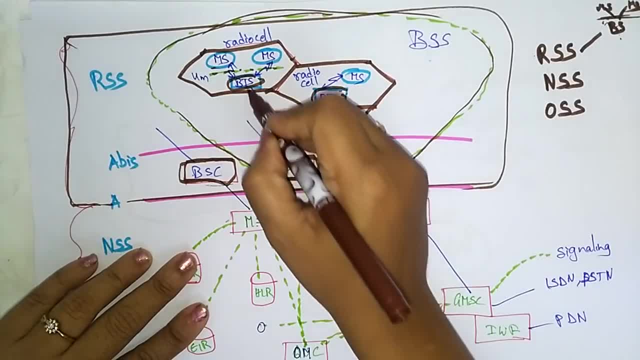 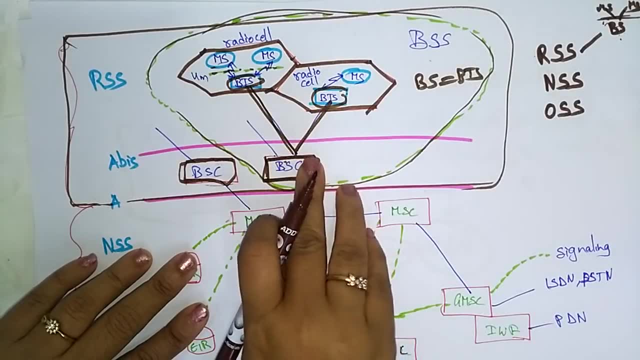 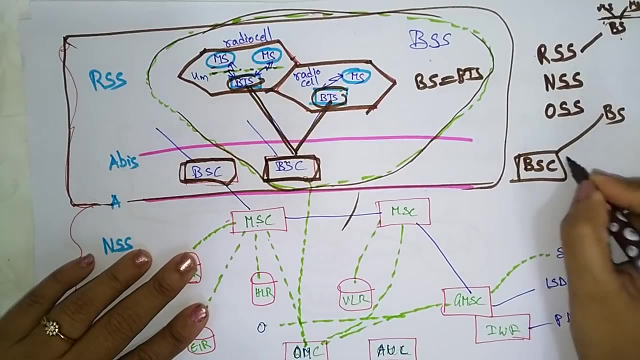 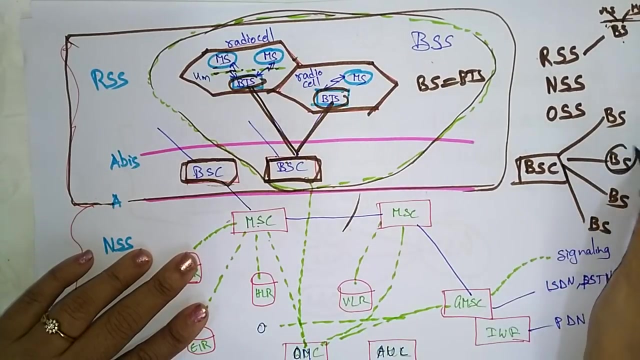 the base station controller is having one or more base stations, bts or bs, both are the same. okay, don't confused so what i said. one base station controller is handling multiple base stations, so it is going to be decided which base station will be sued for which call. 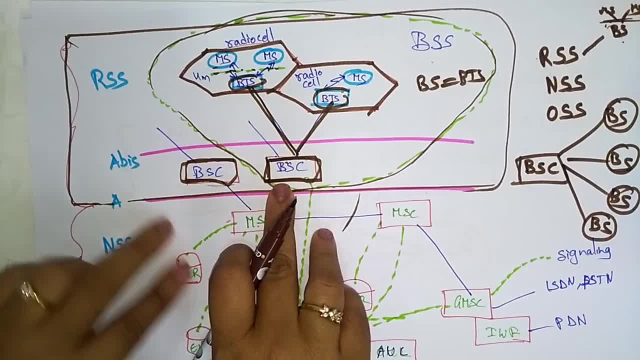 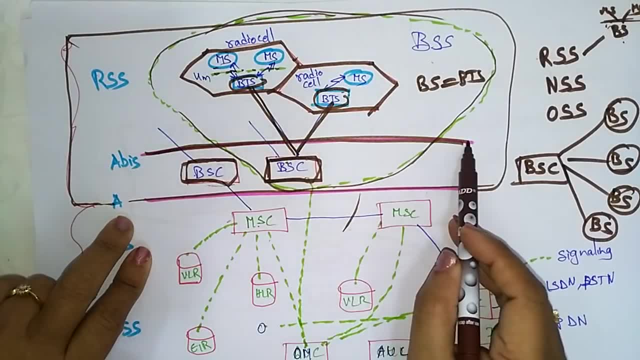 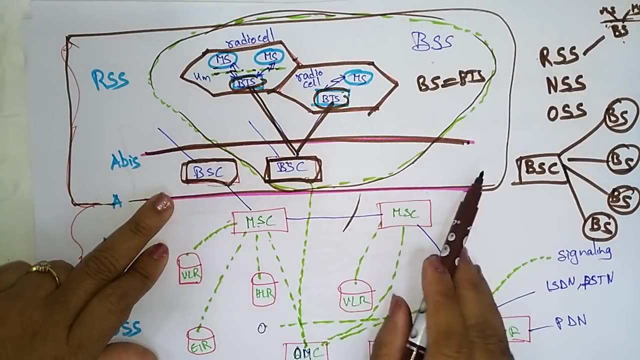 that is controlled by base station controller. so there is an interface between the base station and the base station controller. that is abis. one interface will be there, okay, and uh, different base controllers will be there. base station controllers will be there. so one base station control is monitoring some cells and another base station controller is 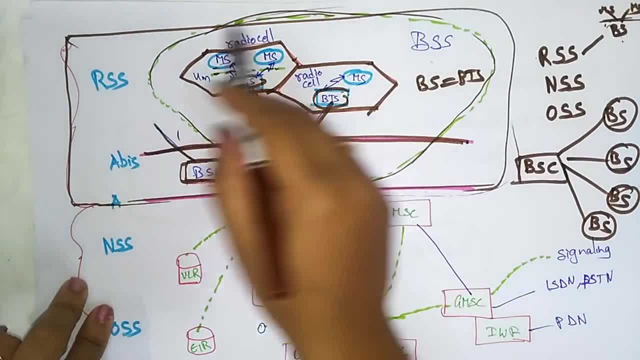 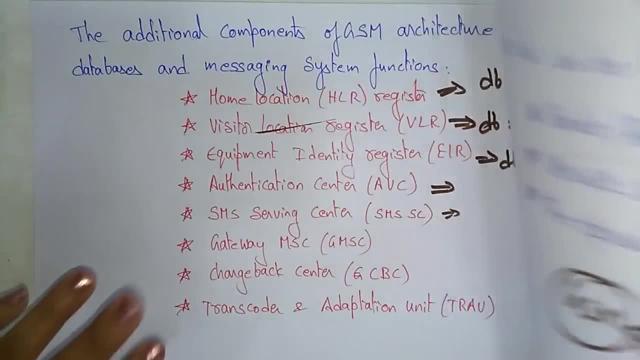 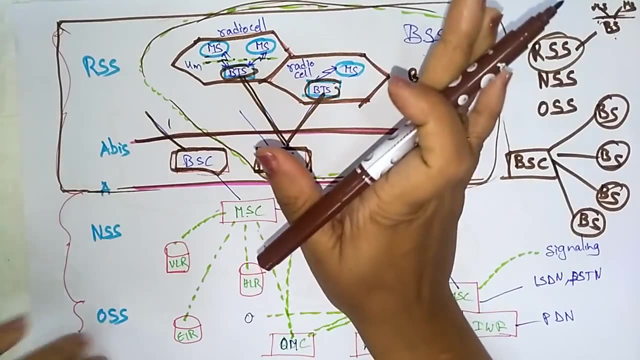 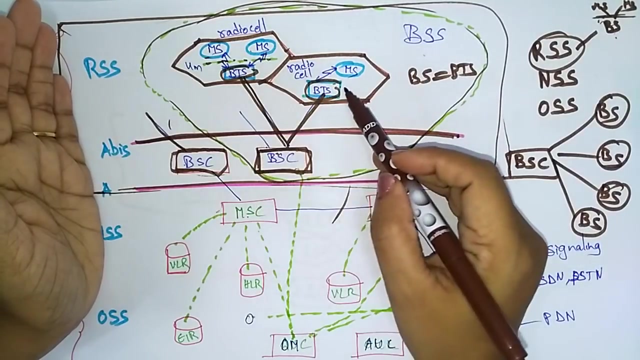 monitoring another cells like that. so this complete structure, you call it as a system, you call it as a radio system switching subsystem. okay, so what it is? radio station subsystem. rss is a radio station subsystem. is it clear? this radio station subsystem, consisting of the radio cells that radio cells is monitor, having different base stations. the base station- 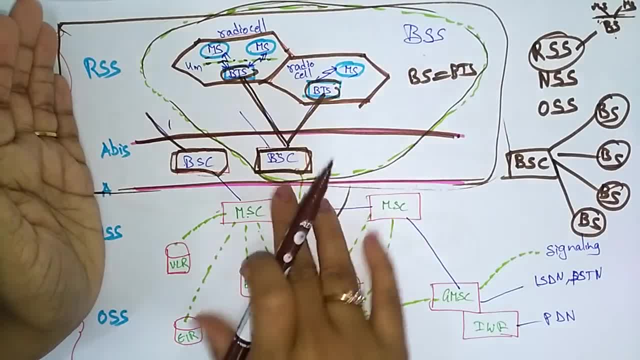 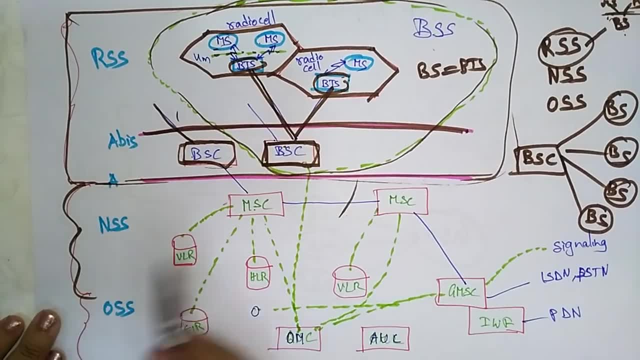 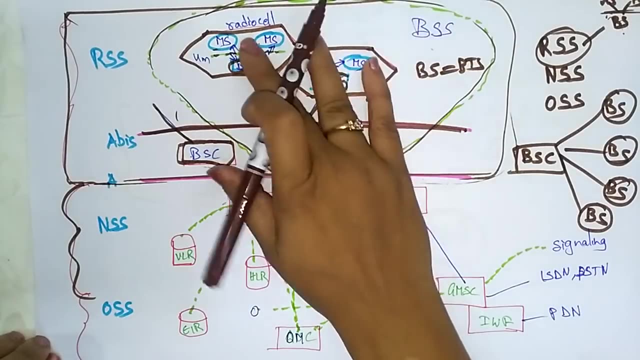 is handling one or more mobile services. all these base stations are controlled by one base station controller. okay, so now let's coming to the next subsystem. so here everything, the connection is established. so this a call, a connection is the base stations- is controlled by the base station base station switching circuit. okay, so. 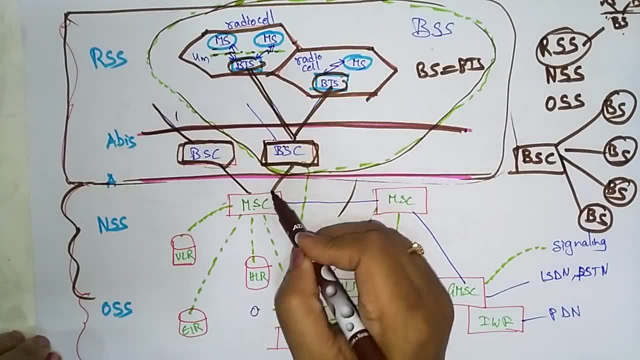 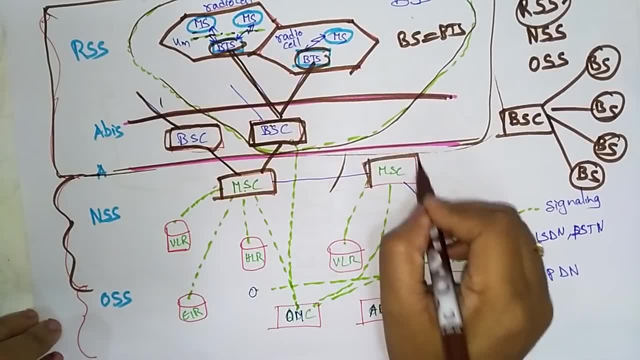 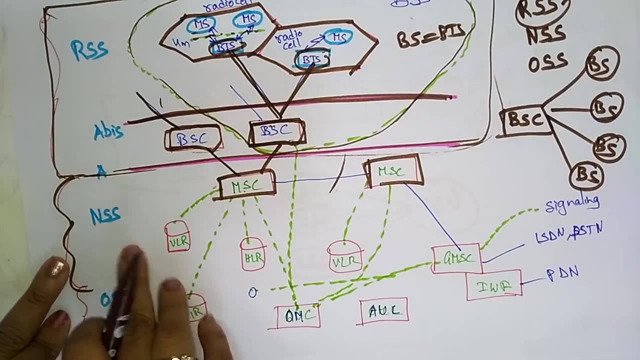 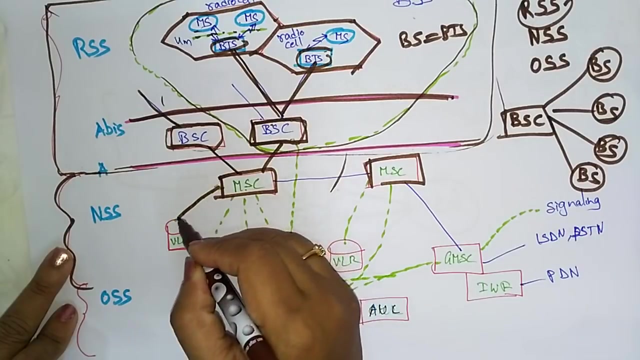 Okay, so this will be controlled by mobile switching circuit. The mobile switching circuit is present in the network subsystem, network switching subsystem. Okay so this mobile switching circuit or mobile switching controller, is handling the VLR visitor location register, EIR, identity register, HLR. 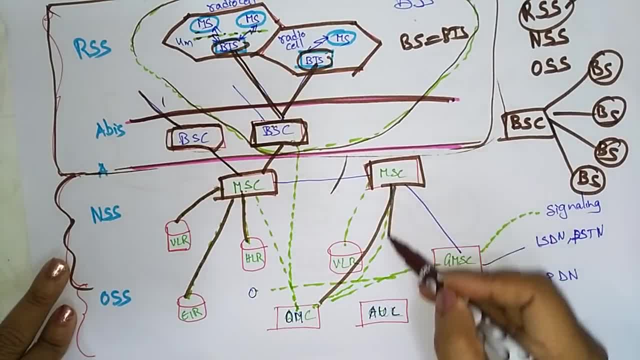 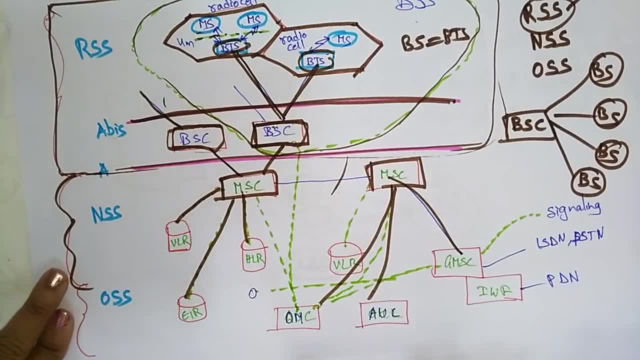 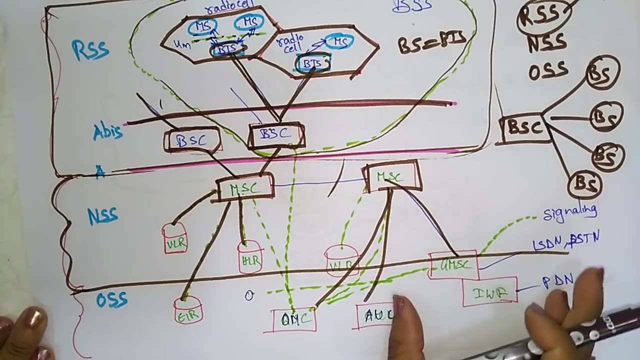 Okay, and all: OM, authentication, GHMC, gateway, IWF. So these are all the terms I will explain clearly, don't be confused. And OSS: the operator Operating switching subsystem consisting of the operations like authentications or the identity of the mobile. 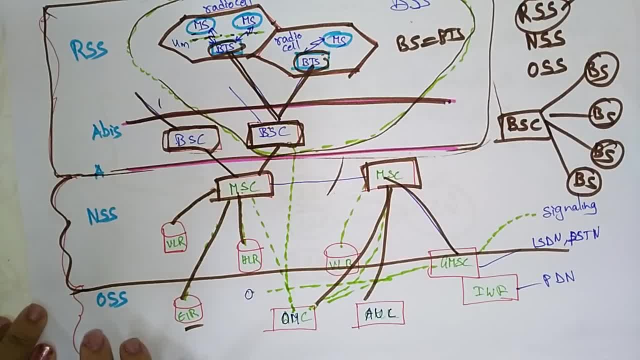 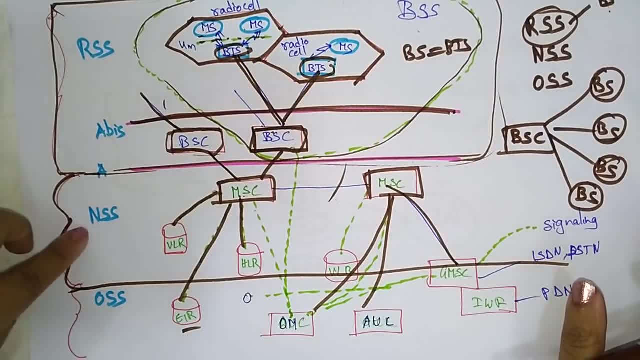 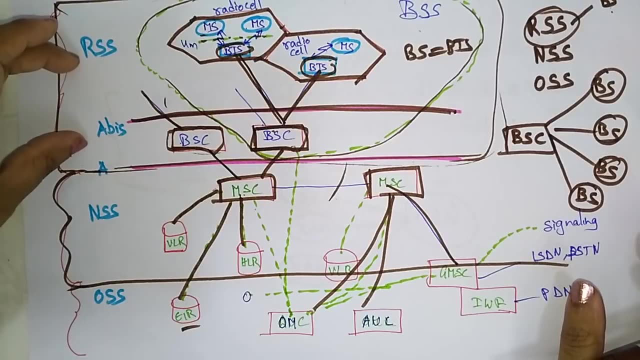 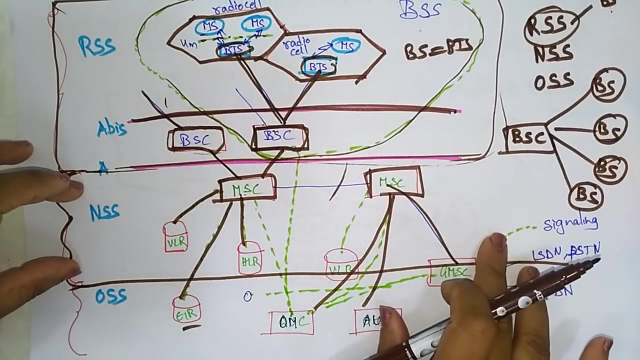 Okay, all that information will be stored in the operating subsystem. So the complete GSM will be divided into radio switching subsystem, network switching subsystem and operating switching subsystems. Okay, so this deals with the cells and the base station controller, And here it is completely about the database, that means the details of the means, the locations of the mobile phone monitor by the mobile switching circuit. 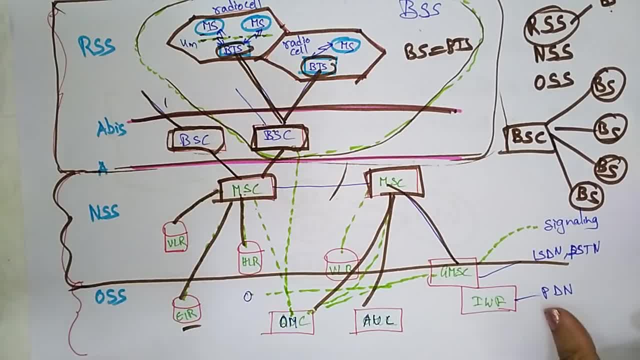 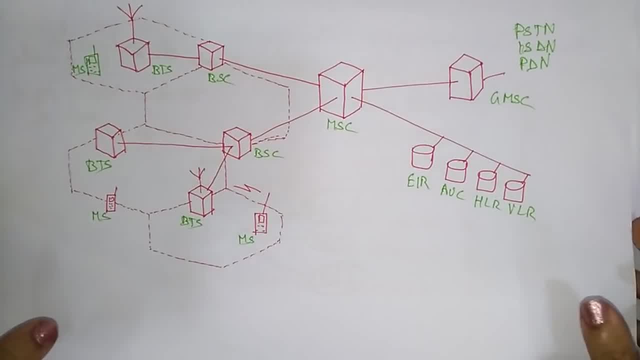 And OSS is having the identity and authentication that you have to be remember. Now let's see what exactly the each terms will be. Before going that, I want to just show you this diagram. So here, one base station is there, BS. 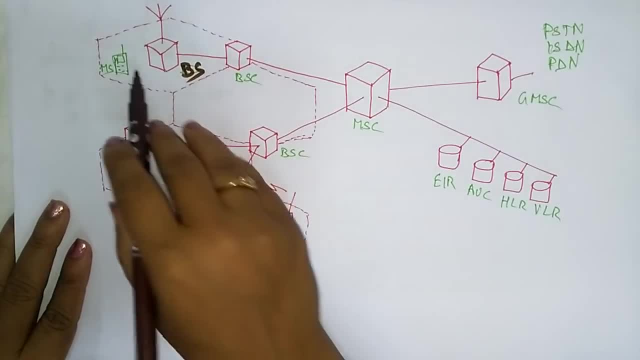 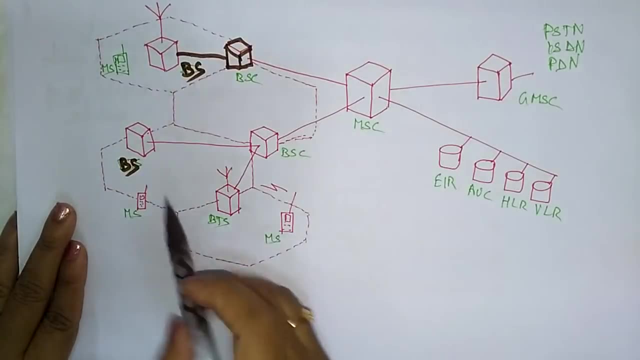 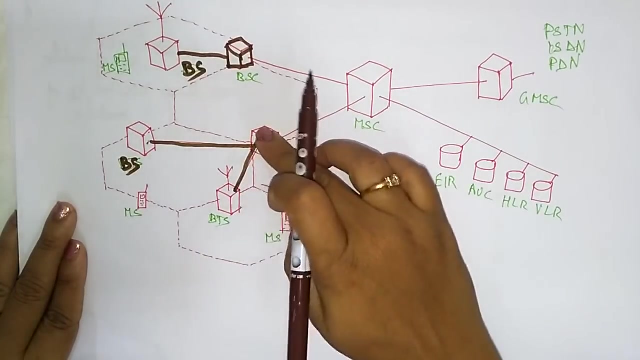 And another base station in this cell And another base station in this cell And this base station is controlled by base station control unit Okay, and this base station is controlled by another base station control unit. So many base stations are controlled. 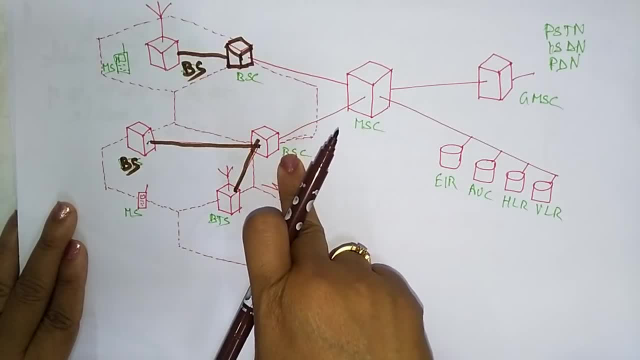 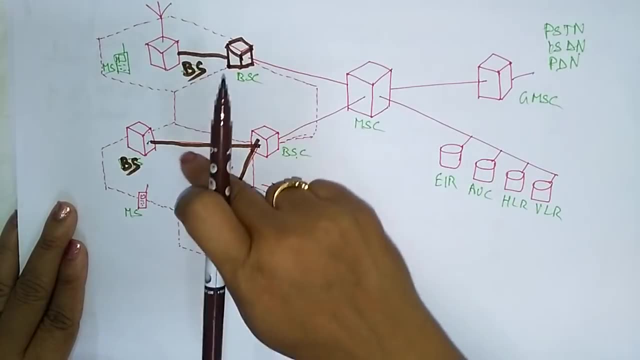 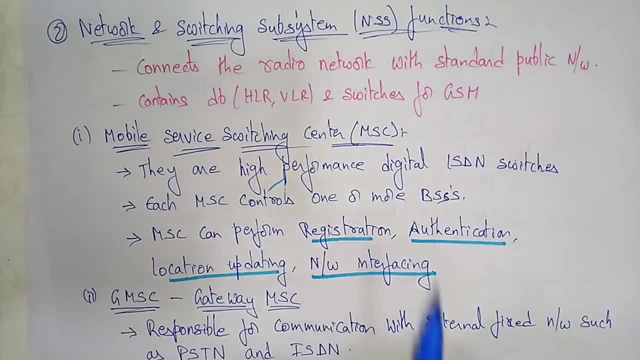 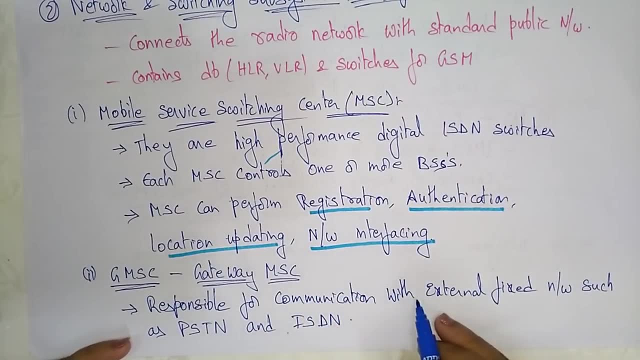 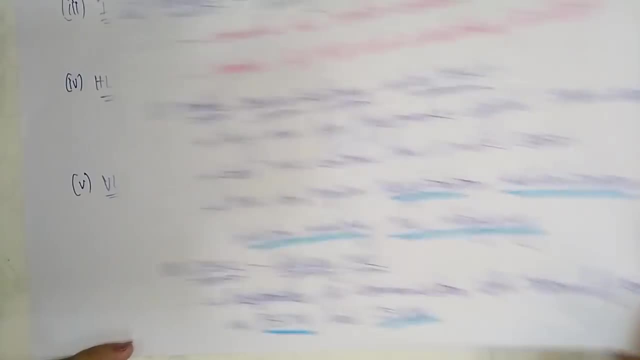 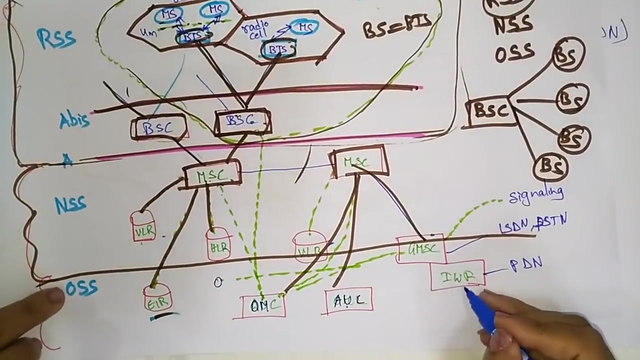 location, updating network interfacing and what is the next term? gmsc, that is a gateway mobile switching center. it is a responsible for communication with external fixed networks such as public switch telephone network and isdn, and the next term that we are having is the iwf. so this is completely. it is in this nss only. 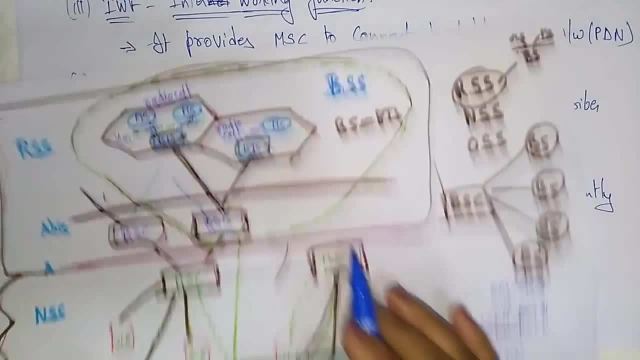 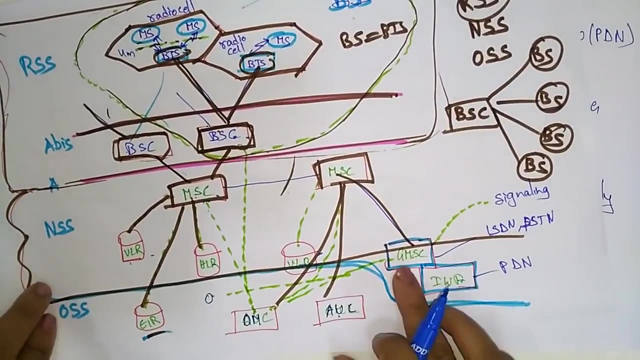 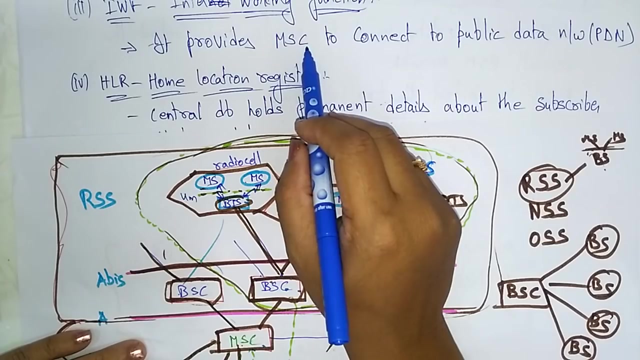 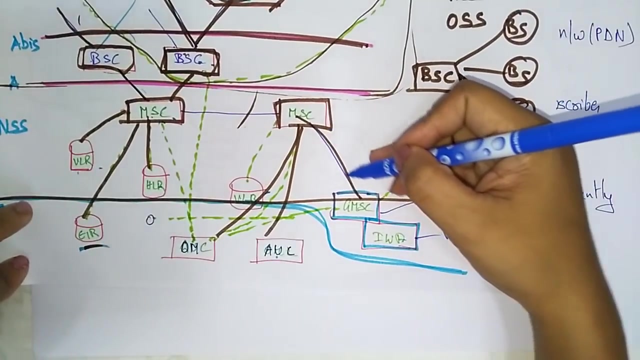 internet working function. this internet working function is attached to the gm gateway mobile switching center internet working function. it provides the mobile switching set center to convert to public data network. okay, so whatever the mobile switching circuit will sense that information that it contains the sense: convert the data into public. 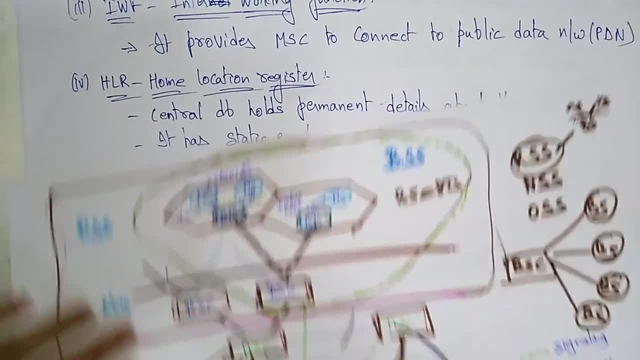 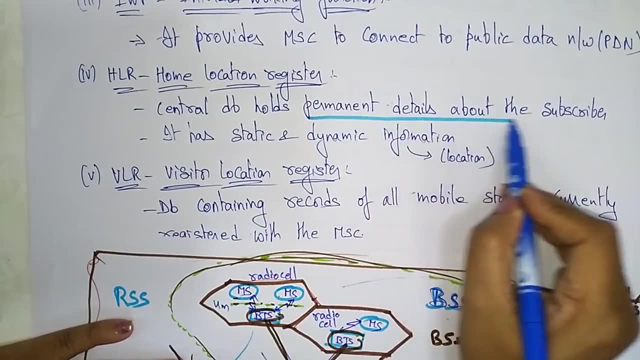 network. so whatever the mobile switching circuit will sense that information, that it contains the sense, convert the data into public data network. next is the home location register. the home location register is a central database holds the permanent details about the subscriber. suppose you are the subscriber and you are a retail subscriber, like that, so your complete 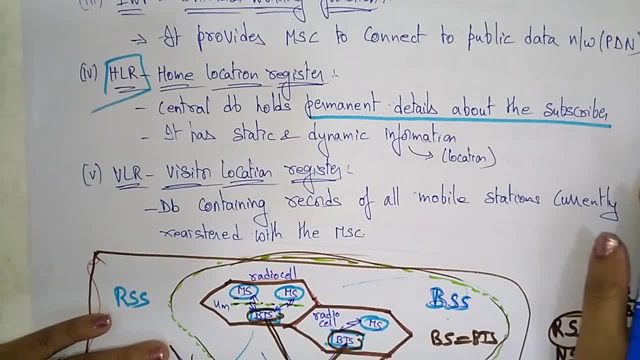 permanent details will be stored in home location register, so it has a static, and the dynamic information is also there. static information regarding your mobile data and your address. permanent information is also there. static information regarding your mobile data and your address- permanent address. everything will be static and the dynamic information is nothing but the location you are shifting, suppose you are at present it in. 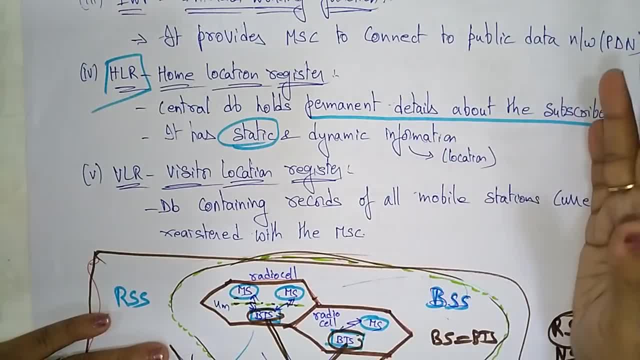 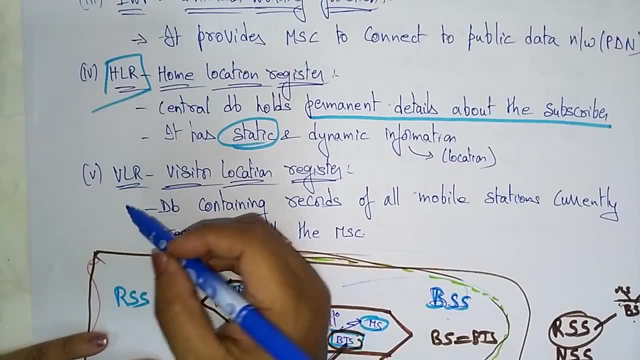 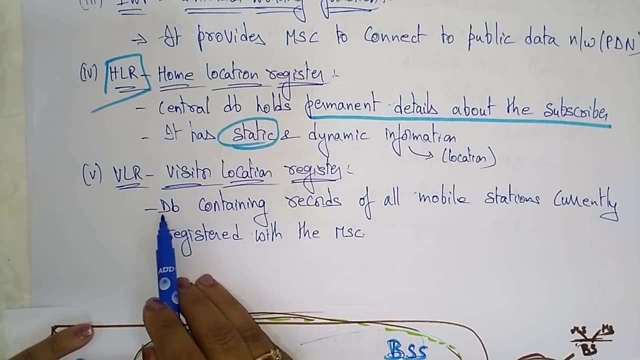 hydropad. suppose you are going to somewhere else, vijayawada. the location is changing, so this look home location register may be a static and the dynamic and in the network switching subsystem vlr is there. so visitor location register. it is also a database. hlr is a central database and this is a database vlr containing records of the